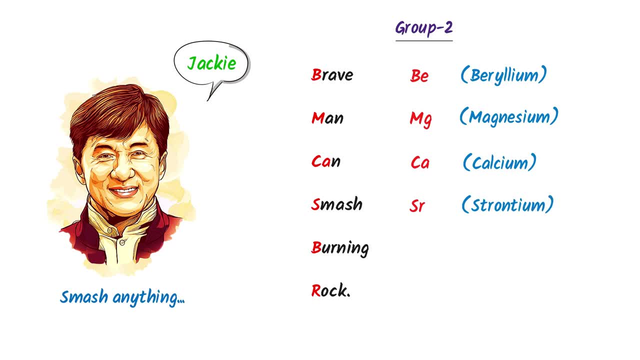 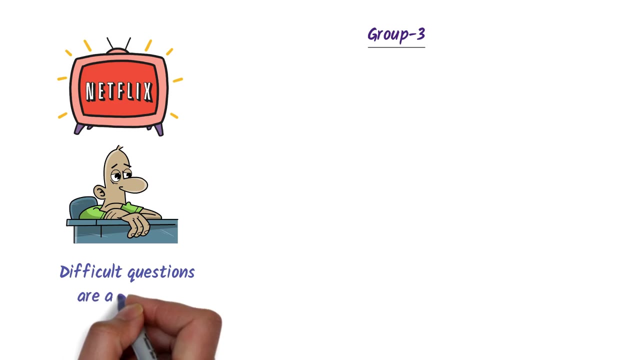 S stands for SR strontium, B stands for BA barium, R stands for RA, radium. Thus, this is the second group of the periodic table. Thirdly, consider Netflix. Let you watch a famous series where difficult questions are answered. 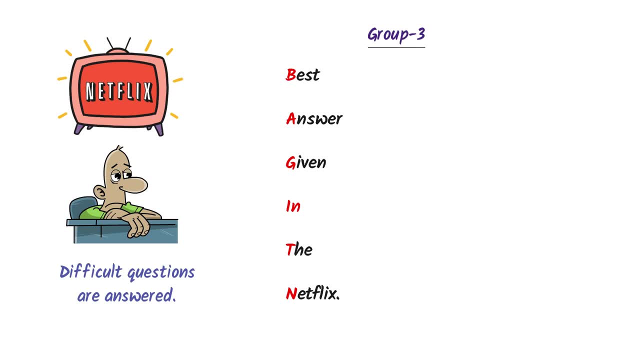 So I say best answer given in the Netflix Here: B stands for boron, A stands for aluminium, G stands for gallium, I stands for endium, T stands for thallium, N stands for nihonium. 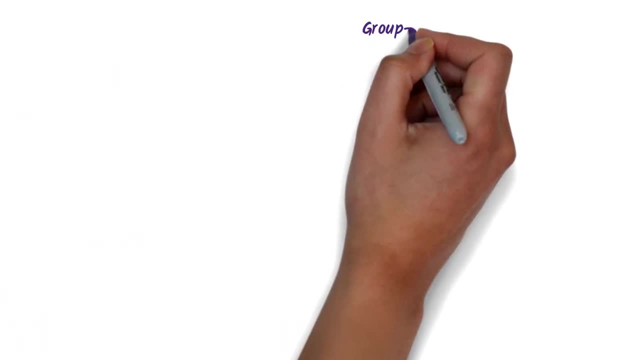 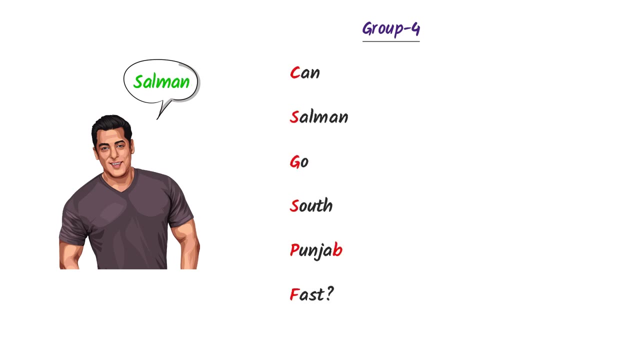 Thus, this is the third group of the periodic table. Fourthly, consider Salman Khan. We know that he is very strong man. I say: can Salman go South Punjab fast Here? C stands for carbon, S stands for Si silicon. 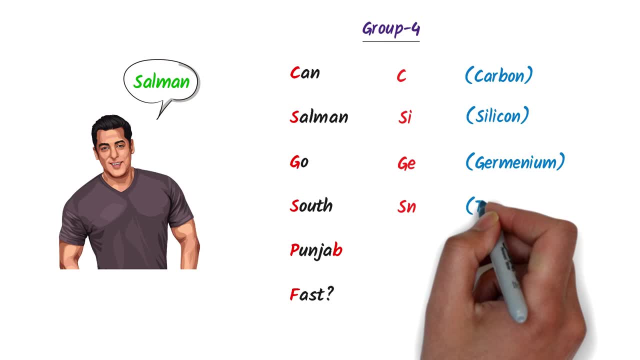 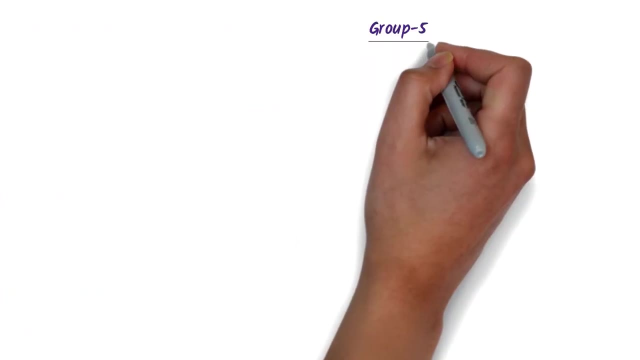 G stands for GE, germane. Here. N stands for titanium. S stands for Sn, which is the symbol of tin. P stands for Pb, which is the symbol of lead. F stands for Fl, which is Fluorium. Thus, this is the fourth group of the periodic table. 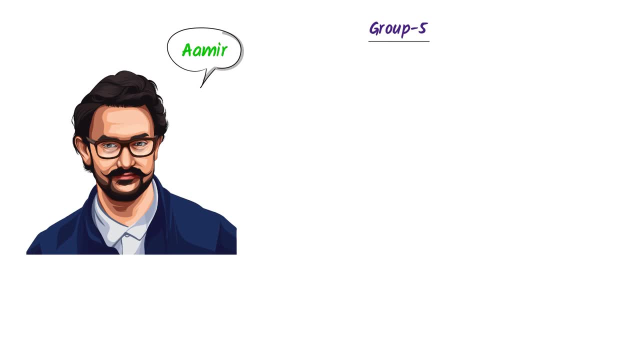 Fifthly, consider Aamir Khan. We all know about the muscles of Aamir Khan. I say: no problem, Aamir Saab builds muscles Here. N stands for nitrogen, C stands for phosphorus, A stands for As, which is the symbol of arsenic. 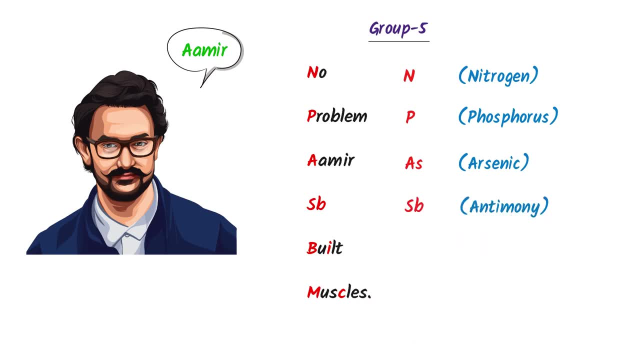 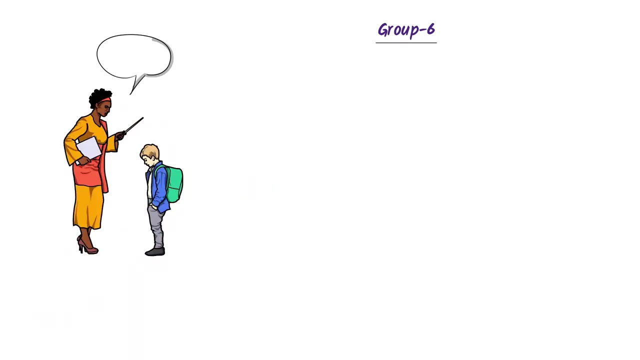 S and B stands for Sb, which is the symbol of antimony, B stands for Bi bismuth, M stands for Mc Muscovium. Thus, this is the fifth group of the periodic table. Sixthly, consider your serious teacher in the school. 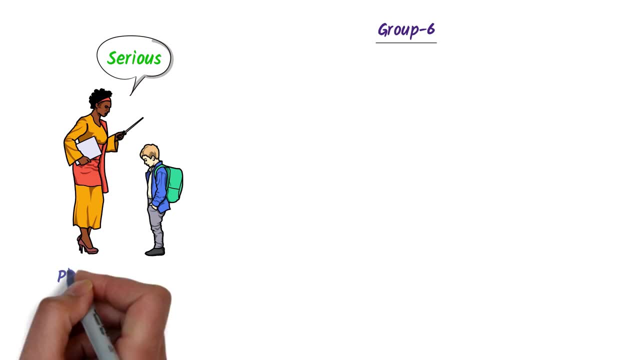 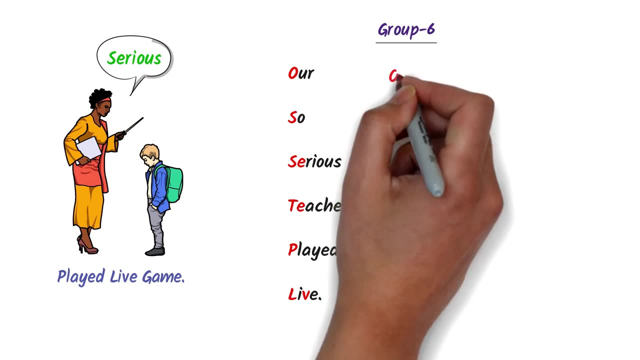 Remember his name and his face. Let he played live game with you. I say are serious teacher in the school. I say are serious teacher in the school, So serious teacher played live Here. O stands for Oxygen, S stands for Sulphur. 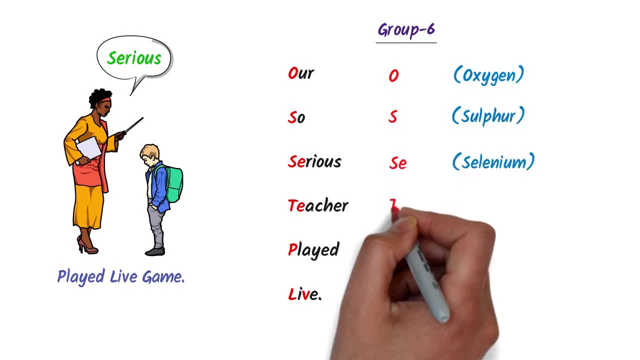 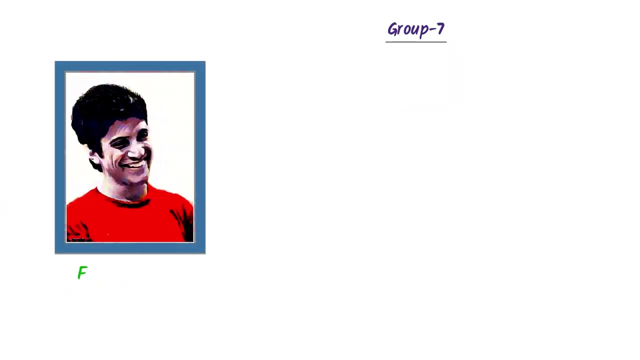 this: Se stands for Selenium, Te stands for Tellurium, P stands for Popilonium L and V stands for LV Livermorium. Thus, this is the sixth group of the periodic table. Seventhly, consider Farhan Akhtar. 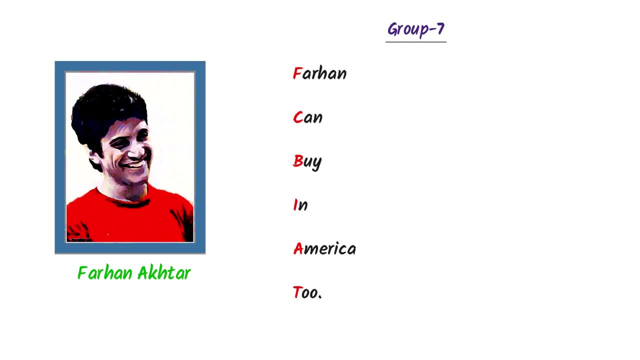 We know that Farhan can buy in America. F stands for Fluorine, C stands for Chlorine, B stands for Bromine, I stands for Iodine, S stands for Estetine. Thus, this is the seventh group of the periodic table. 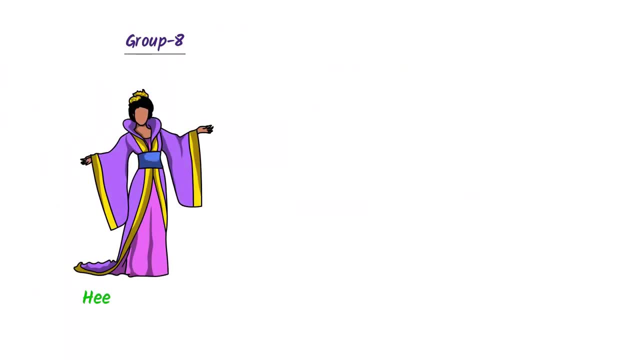 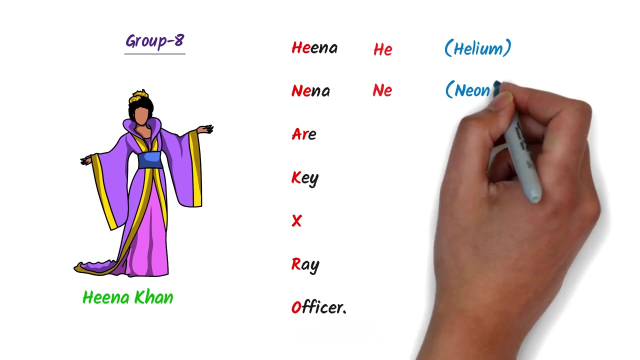 Eightly. consider Hina Khan, and we know that she is famous Bollywood actress. I say: are key X-ray officer Here. H? E stands for H E. X stands for H E- Helium. N? E stands for N E- Neon. 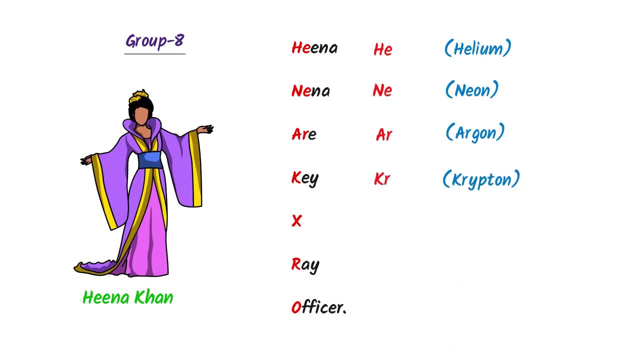 A. R stands for Argon, K stands for K R Krypton, X stands for X E Xenon. R stands for R N, Radon and O stands for O G Ognacium. Thus, this is the eighth group of the periodic table. 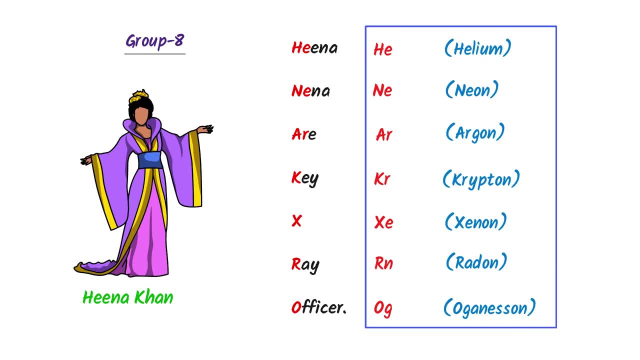 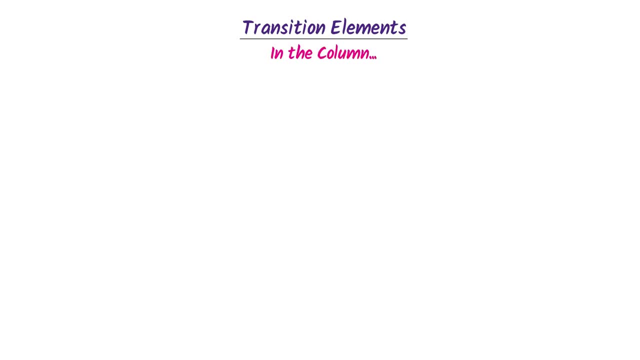 So we have learned the main groups are eight groups of the periodic table. Now we will learn about transition elements. Remember that I write them in the column. Let consider science team of your school. I say science team, visit cancelled. friends cannot come zoo. 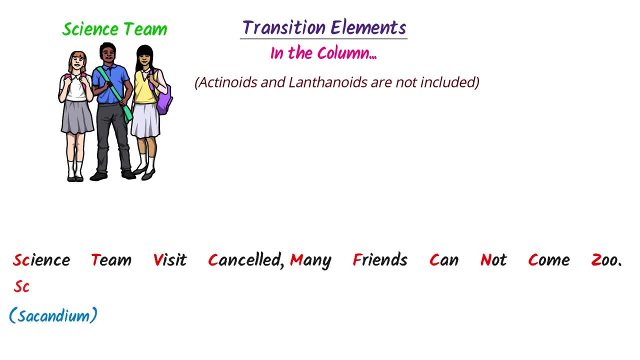 Here: S C stands for S C Scandium. T stands for T I Titanium. V stands for V. Vanadium C stands for C R. Chromium M stands for M N. Manganese F stands for F E. Iron C stands for C O Cobalt. 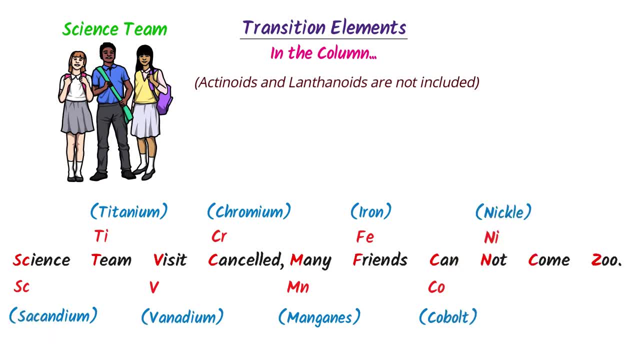 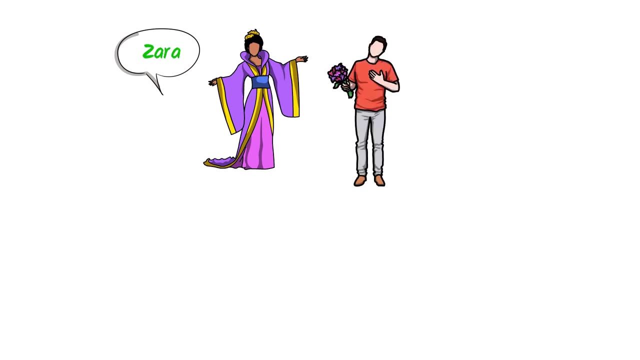 N stands for N I. Nickel C stands for C U. Copper Z stands for Z N, Zinc. So this is the first column of transition elements. Secondly, consider a famous actress, Zara Noor. I send her some flowers, but there is a problem. 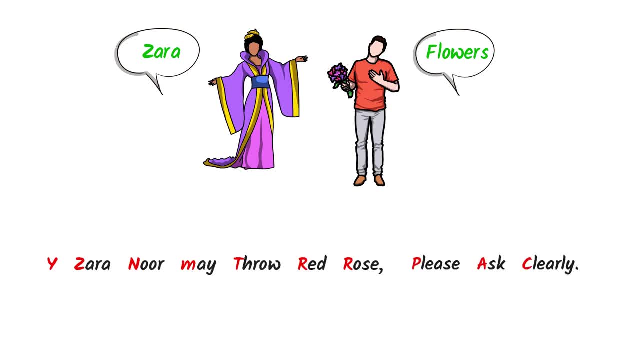 Why Zara Noor may throw red rose. Please ask clearly Here. Y stands for Yttrium, Z. R stands for Zirconium, N stands for N B. Niobium. M stands for M O, Molybdenum. 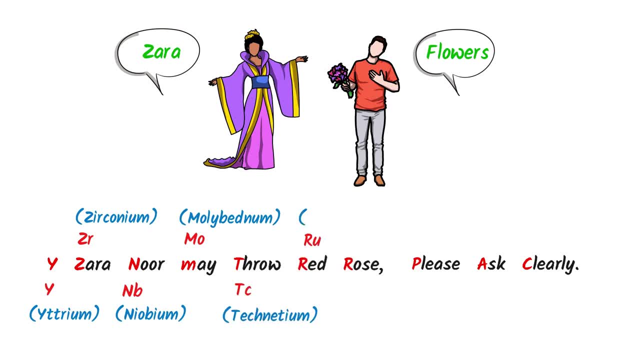 T stands for T C. Technetium. R stands for R U. Ruthenium. R stands for R H. Rhodium. P stands for P D. Palladium. A stands for A G, which is the symbol of silver. Z stands for C D, Cadmium. 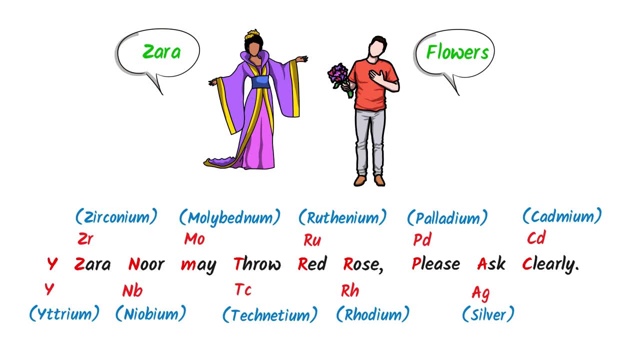 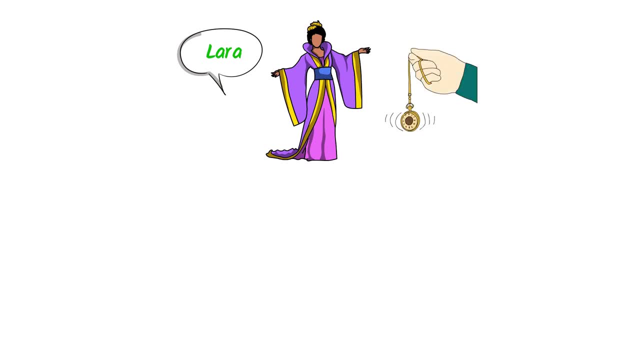 So this is the second column of the transition elements. Thirdly, consider a famous actress, Lara Let. she is making noise while watching a movie. I say Lara, half time well, run. oscillating iron produces R? U High. Here L stands for L? U Lutetium. 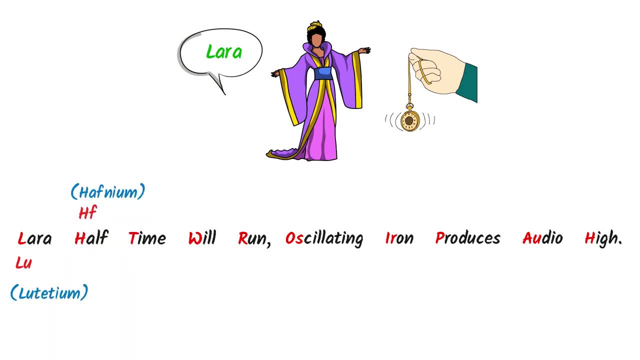 H and F stands for H, F. Hafnium. T stands for T A Tentulum. W stands for W, which is the symbol of tungsten. R stands for R, E, Rhenium. O S stands for O S, Osmium. 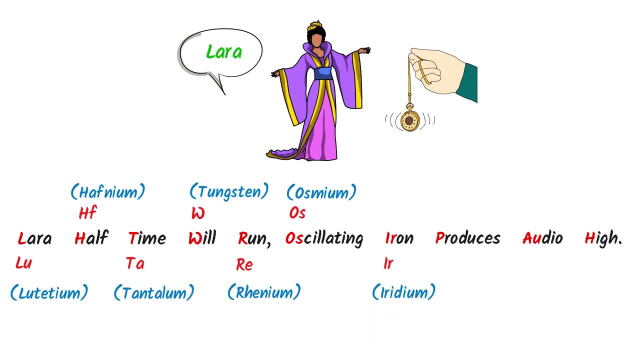 I R stands for I R, Iradium. P stands for P, T, Platinum, A U stand for A? U, which is the symbol of the gold. H and G stands for H, G, which is the symbol of the mercury. Thus, this is the third column of the transition elements. 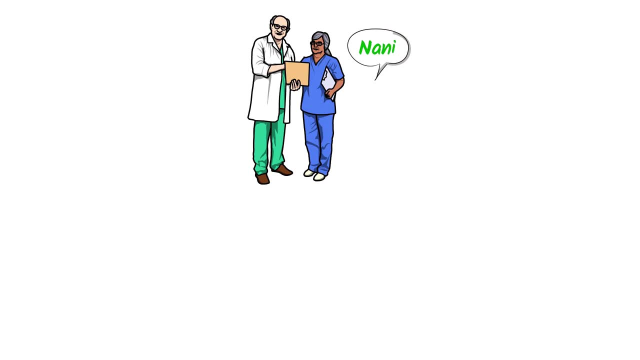 Fourthly, consider your old grandmother Let, she is very sick. She says that low result does show bad health. My doctor repeats it again Here: L stands for L R, Laurentium. R stands for R F Rutherfordium. D stands for D B, Dognium. 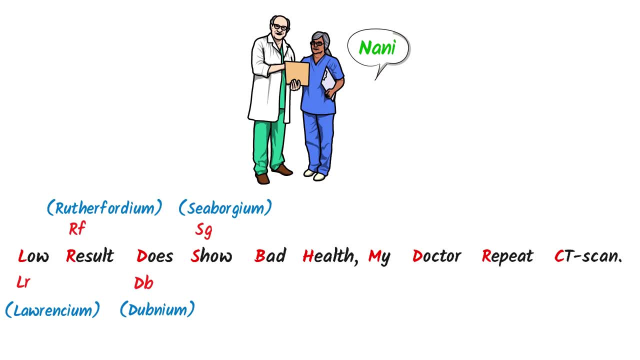 S stands for S G Ciborium. B stands for B H Borium. H stands for H S Hesium. M stands for M T. Minorium D stands for D S Dumpstadium. R stands for R G Rhongium. 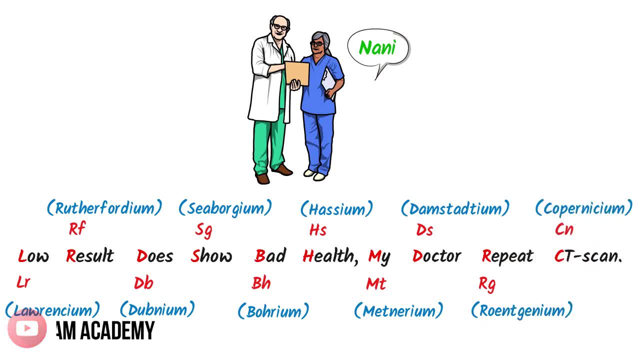 C and N stands for C, N Copernicium. Thus, this is the fourth column of the transition elements. I hope that using this trick, you can easily memorize the periodic table.